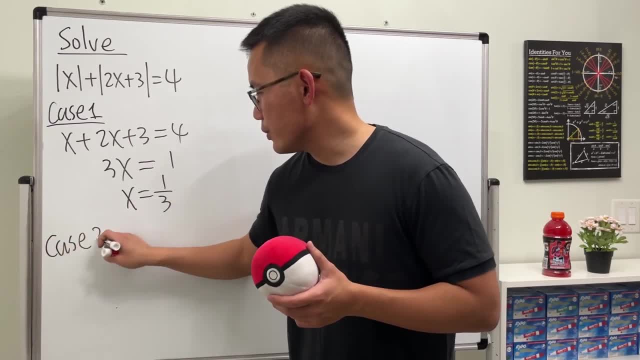 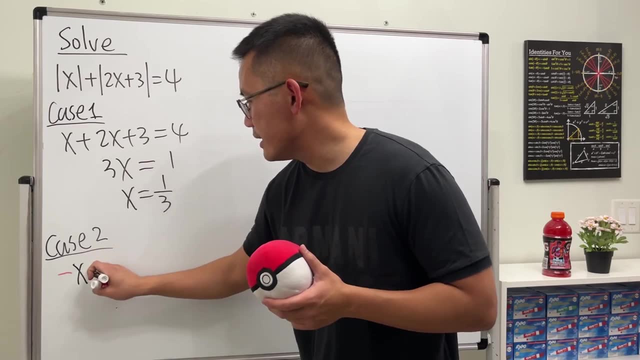 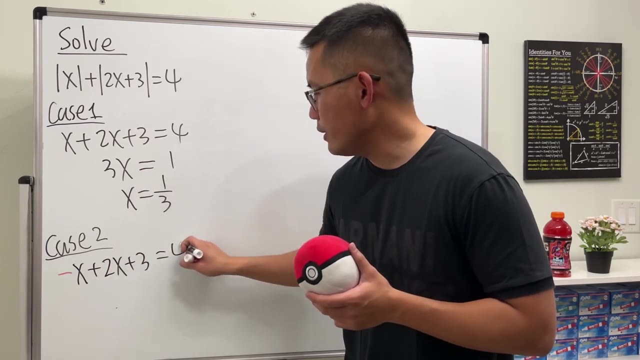 3.. All right, so that's case one. Case two: perhaps let me negate this one right here. first, take out the absolute value and we get negative x and then plus. we keep this positive and we have 2x plus 3 and that's equal to 4.. Okay, this right here will give us x minus 3. on both sides, we get 1. All. 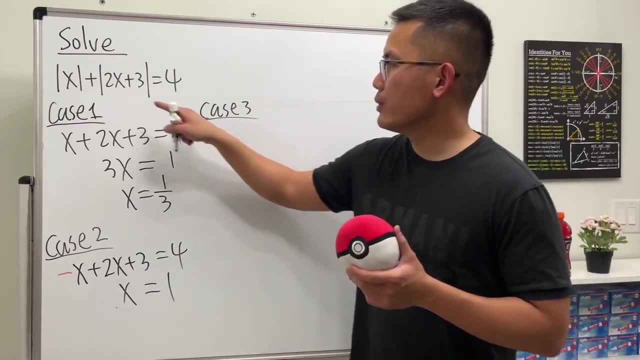 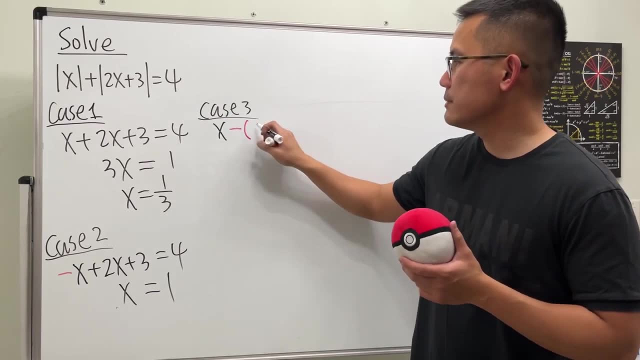 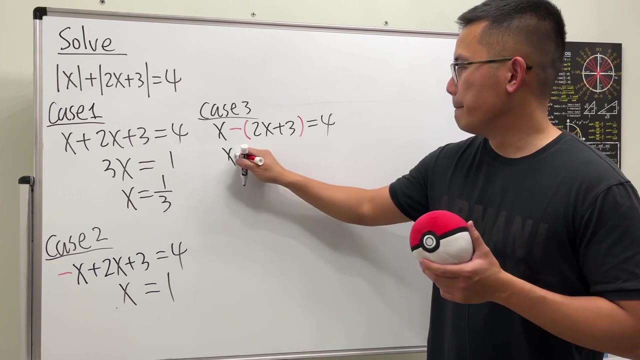 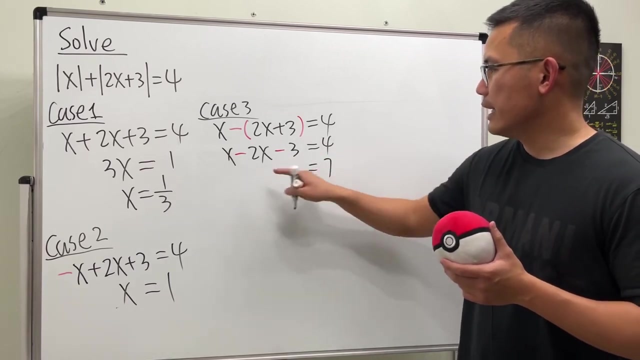 right then case three: I'm going to keep that as positive and then negate that after we take out the absolute value. so we have x and then, minus parentheses, 2x plus 3, and then that's equal to 4.. So, right here, we get x minus 2x, and then minus 3, it's equal to 4. that will give us 7 and this and that will give 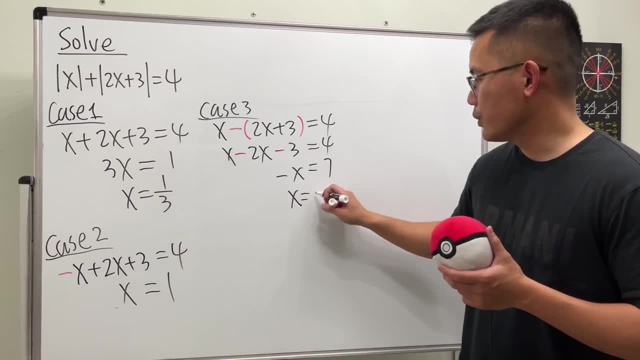 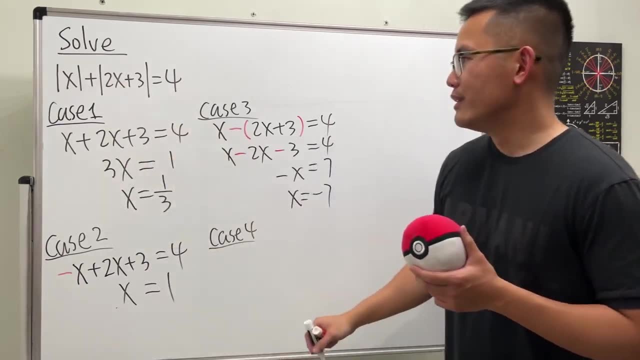 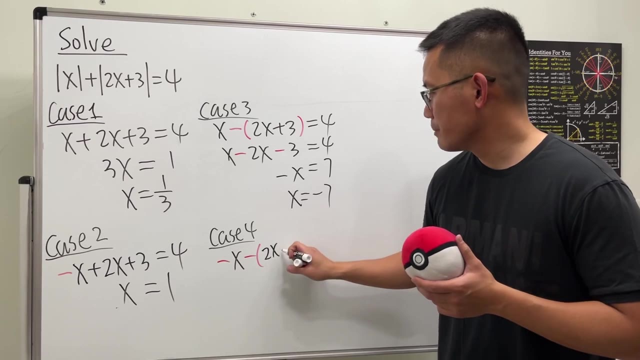 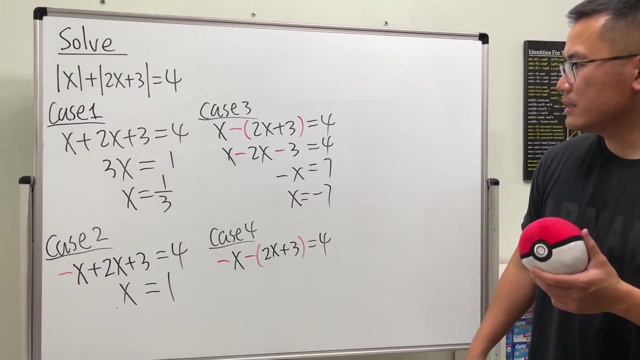 us negative x and divide it by negative 1 x is equal to negative 7.. Lastly, case 4: I'm going to negate both, so we get negative x and then negative parentheses, 2x plus 3, and then that's equal to 4.. All right, so let's see what we will end up. 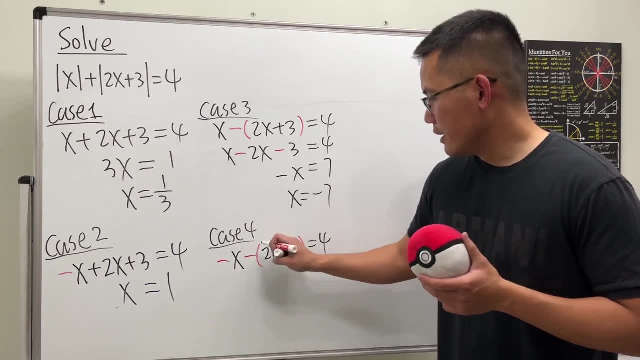 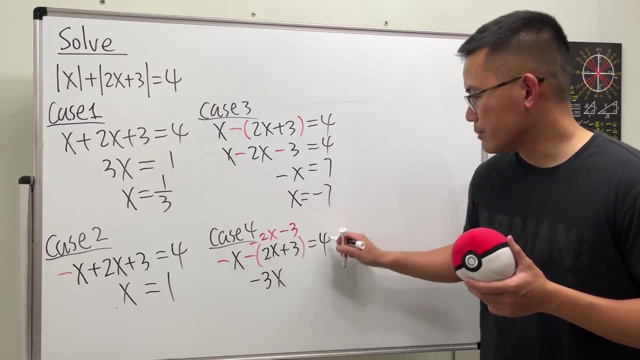 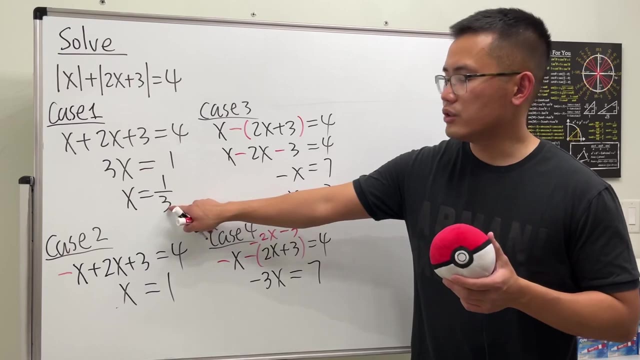 with: Okay, this is going to be negative 2x minus 3.. All right, so that will give us negative 3x, and and then add the 3 on both sides. this is going to be 7. yeah, so this is not just the negation of that, you see, because that's a negative 3, we add the 3 on both. 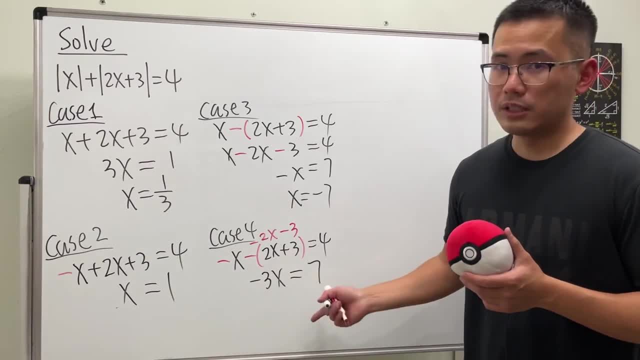 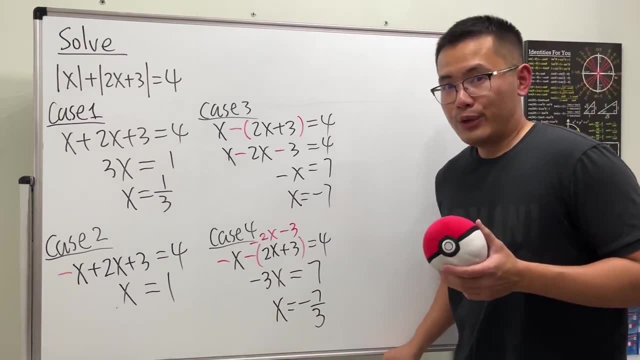 sides, so that's 7, and then what we are going to do is divide both sides by negative 3. so this right here, X is equal to negative 7 over 3. Wow, look at that. it looks like we have four answers, but no, only two of them are legit, so we just 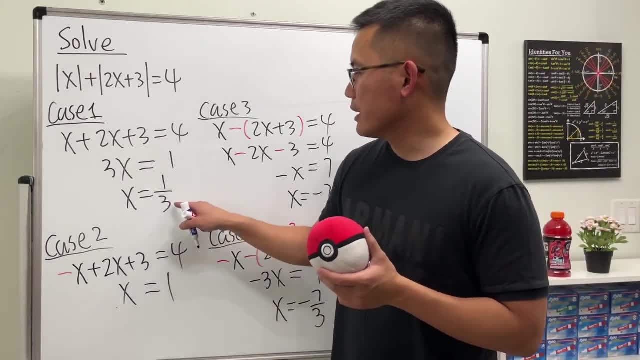 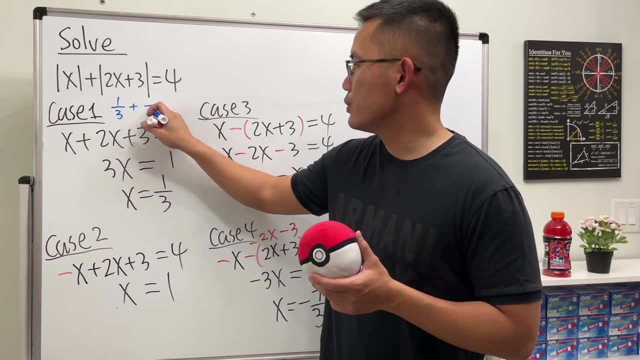 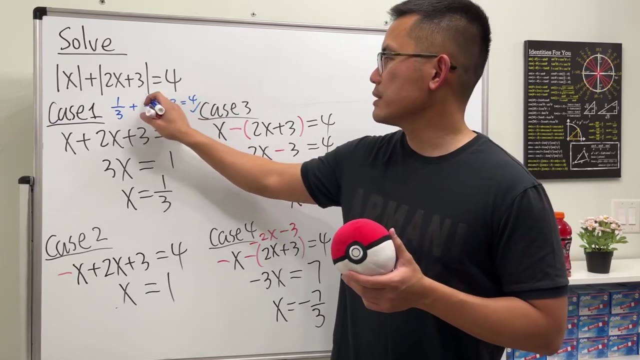 have to plug in and check. so check case one: plug in 1 third in, here we get 1 third. and then plug into here we get plus pretty much 2 thirds and then plus 3, so that's 1 plus 3, which is 4. so this right here does work: absolute value. 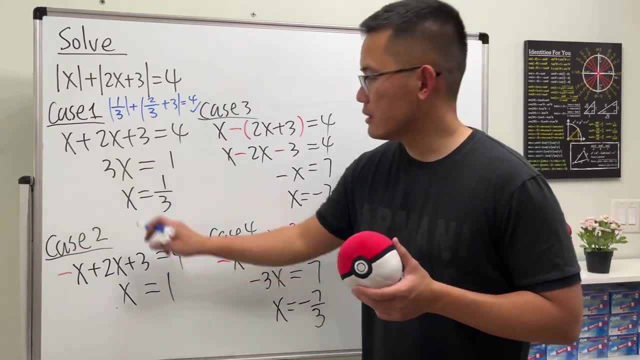 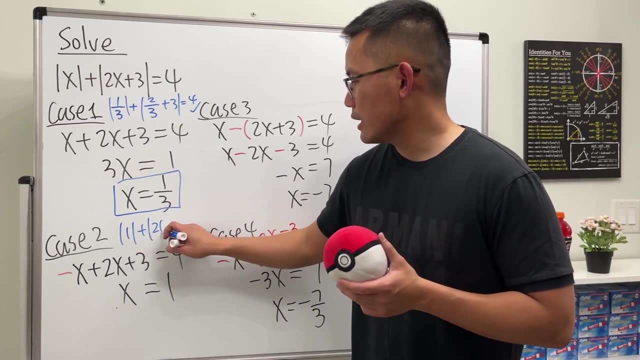 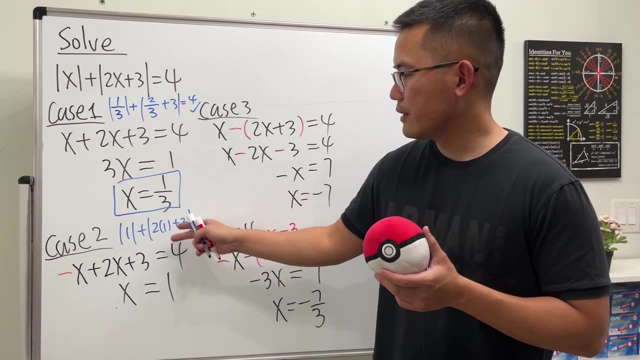 technically, but everything positive doesn't matter. so this right here does work. plug in 1, we get 1 in the absolute value plus 2 times 1 plus 3. have a look, this is 1, but this is 2, 5, 1, that's 6. so no, we don't want that, so this is not yeah. 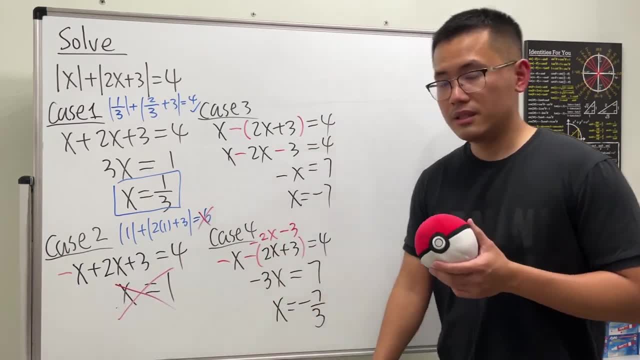 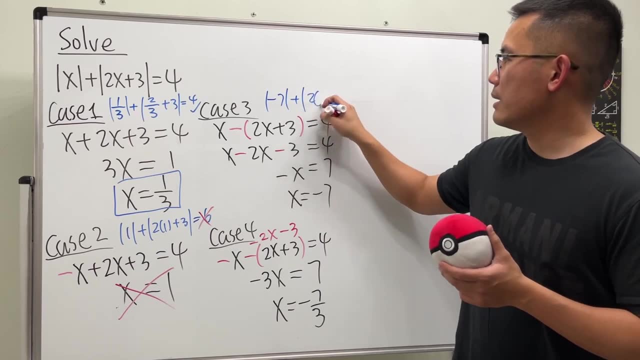 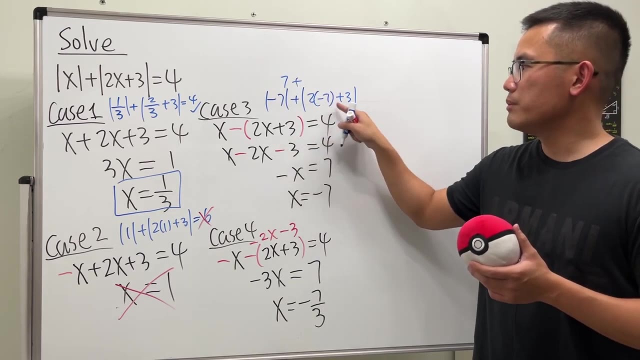 so this is actually not the answer. yeah, plug in negative 7 to there. we get negative 7 in the absolute value, and then plus 2 times negative 7, and then plus 3. this is 7 plus this is negative 14, plus dies negative 11. so it's plus 11. so 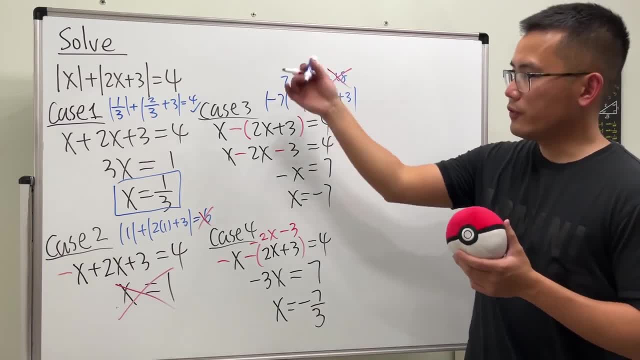 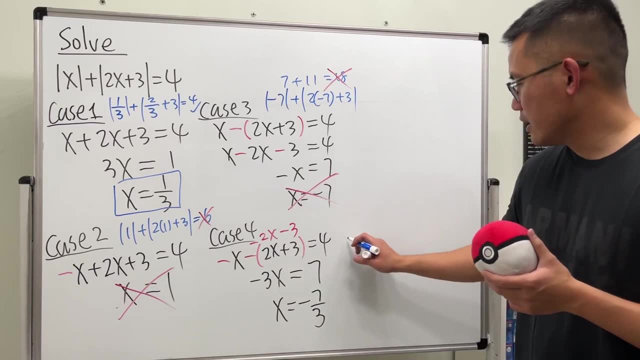 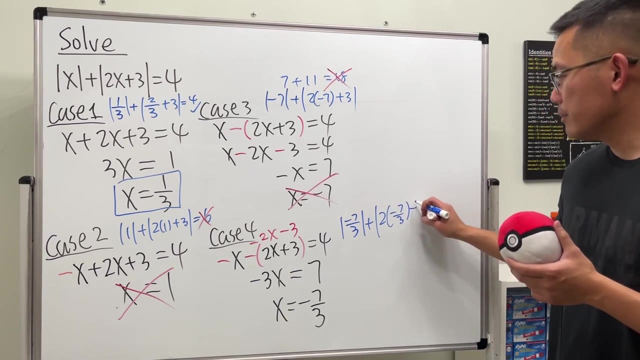 that's 18. that's not what wrong. now we want 4. so negative 7 is not the answer either. plug in negative 7 over 3 into there, so we will get absolute value of negative 7 over 3 plus 2 times negative 7 over 3 and then plus 3, so that's. 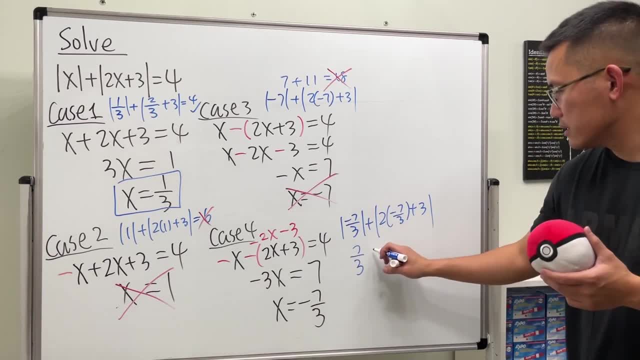 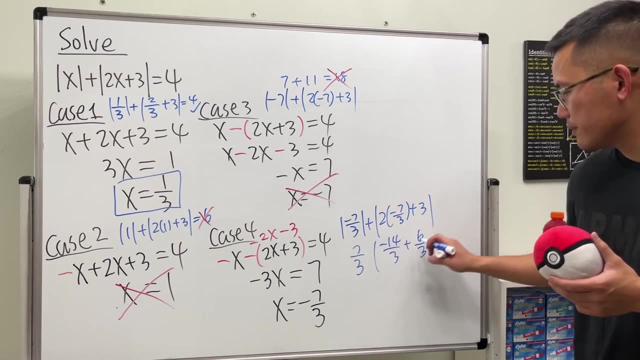 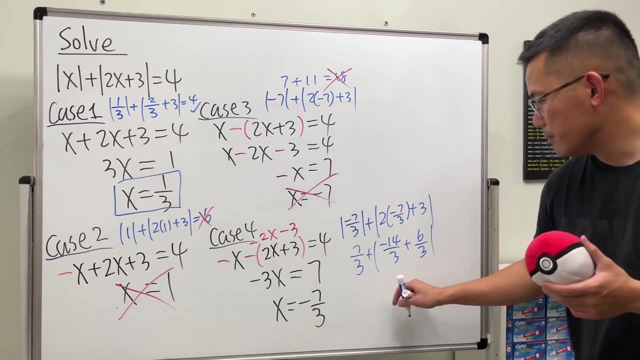 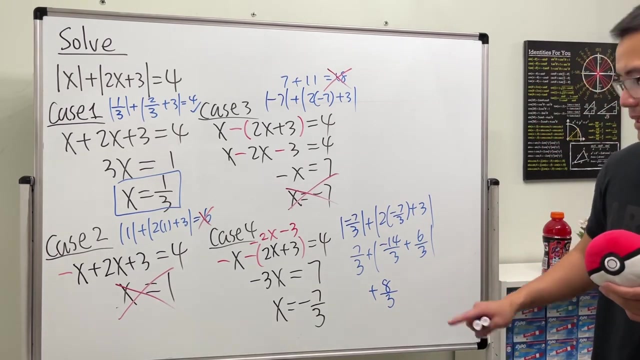 positive seven over three, and this is okay, be really careful. this is negative 14 over 3 plus 6 over 3, absolute value, so that's 8 over 3.. negative 8 over 3, but after that becomes plus 8 over 3.. oh no, sorry, my bad, this is not 6.. 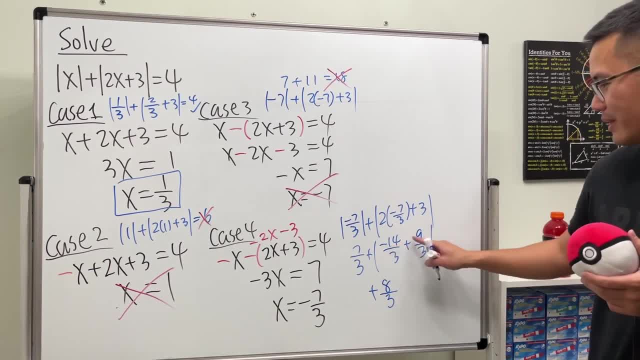 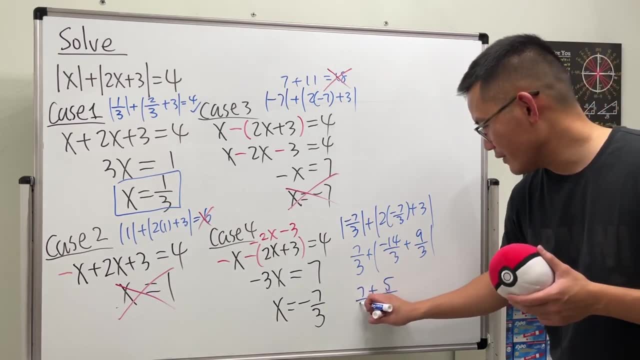 3 is equal to 9 over 3, so this right here will give us negative 5 over 3. by the absolute value becomes positive 5 over 3, and this is 7 over 3, so it's 12 over 3, so we will end up with 4, so it 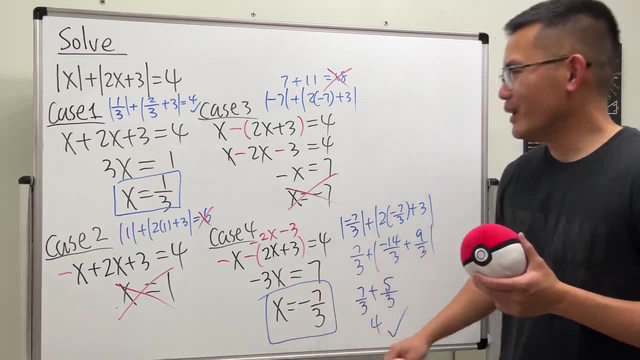 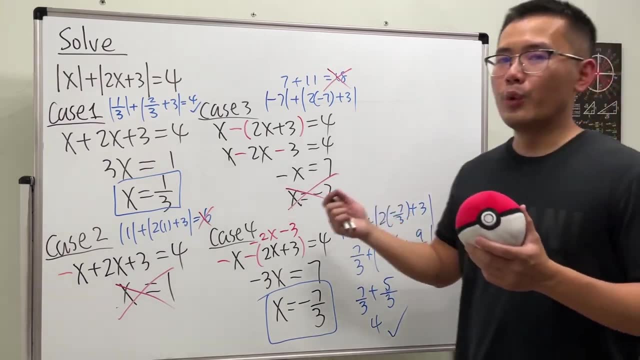 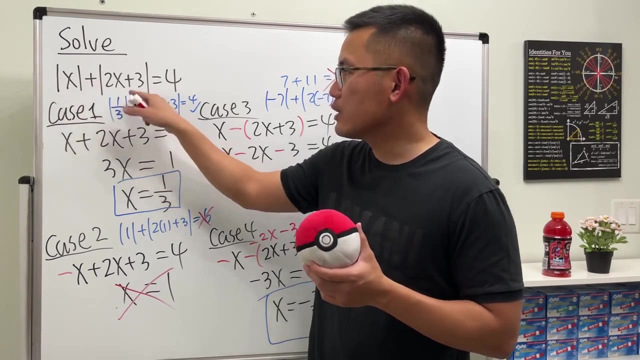 checks. so this right here is also the answer. so, as you can see, we only have two answers. all right, so be really, really careful when we are solving, uh, double absolute value equations. especially we have the absolute value plus another one is equal to a number. all right, so i'm going to give. 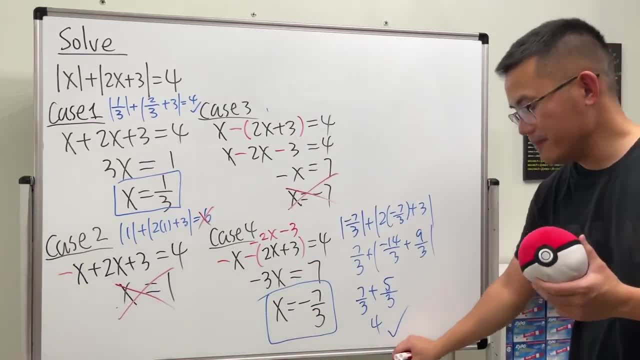 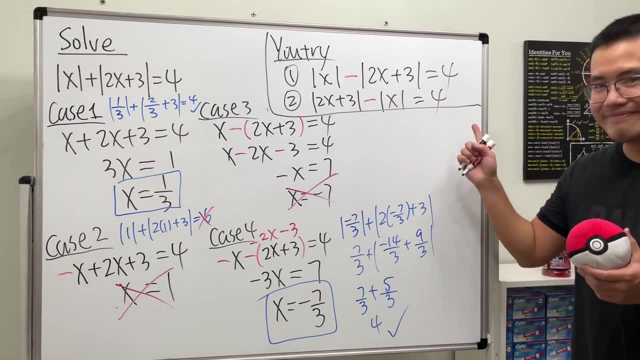 you guys, two questions for you guys to try ready. very similar, so go ahead and try these two questions and comment your answers down below.